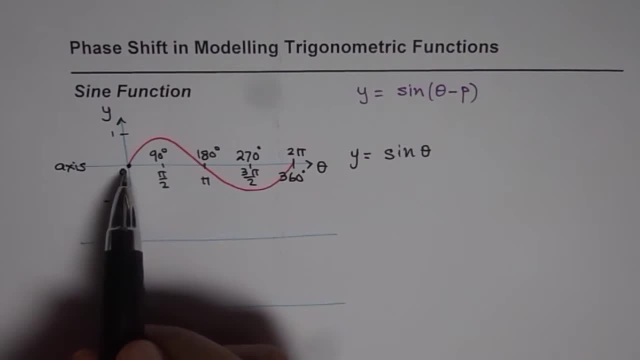 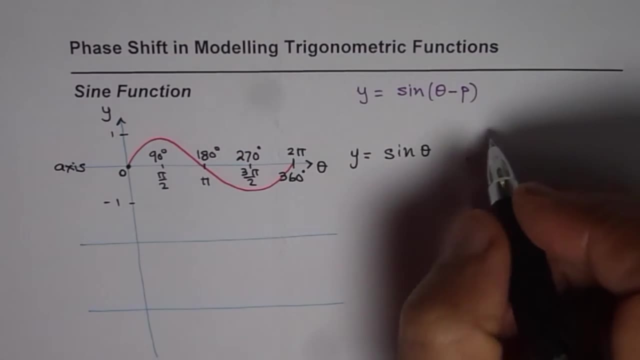 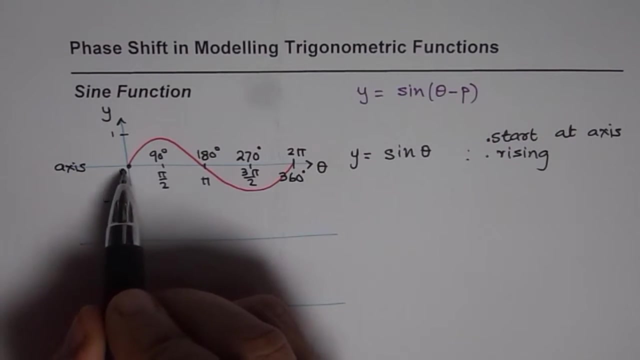 And now we have a particular point from where we have a sine wave which starts from the axis and it is rising. So we are looking for two things: Start at axis and second thing is rising. These two things help us to locate the starting point from the sine wave and then we get our phase shift. 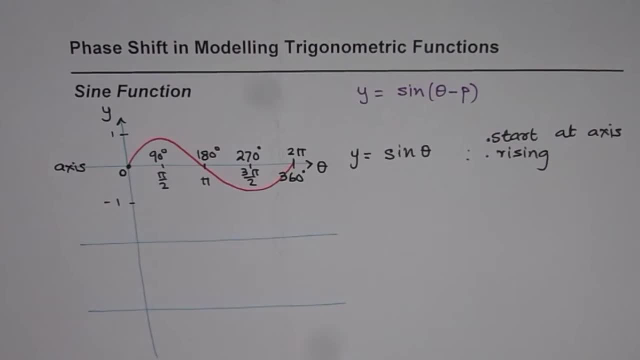 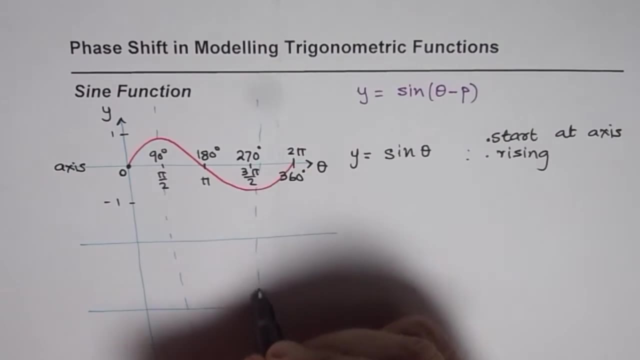 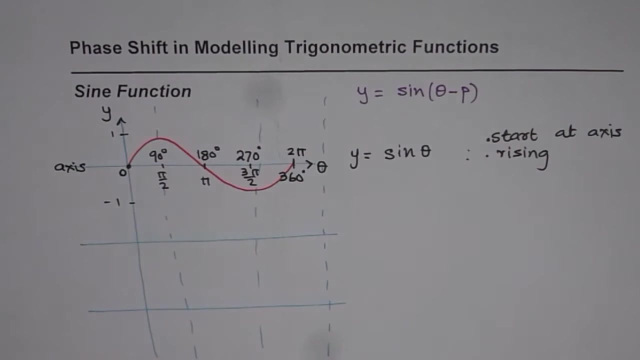 So that is the key thing to do, Which we need to consider in these diagrams. So let me now draw the second sine wave for you. Now, in this sine wave, what I will do is I will shift it by 90 degrees to the right. Okay, So what I'm trying to say is that this sine wave, I am shifting. 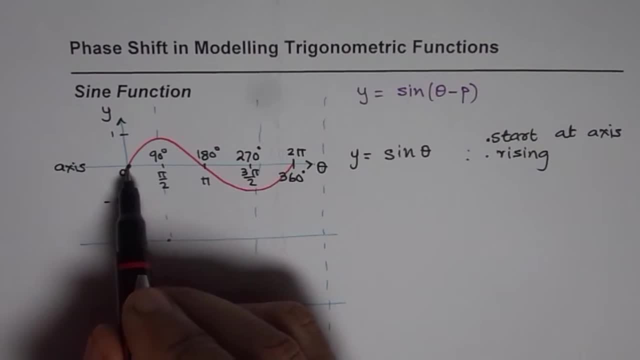 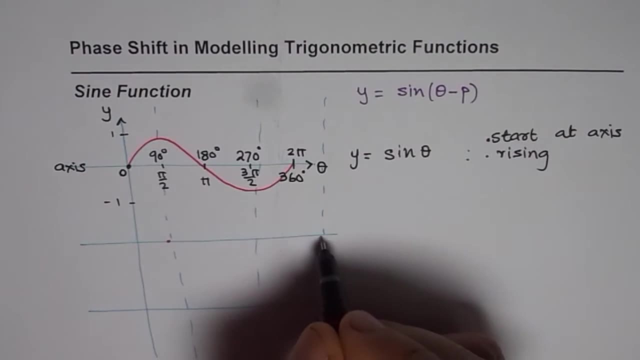 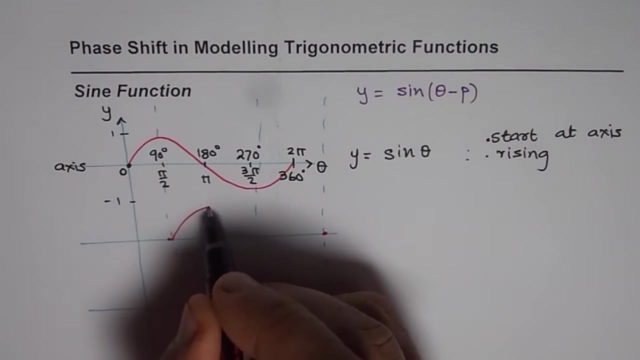 Starting from here. instead of 0 being at 0, 0 on the axis, I am starting my sine wave here, and this sine wave Will now end up 360 plus 90 degrees, since the time period is same for the sine wave. So let me just approximately. 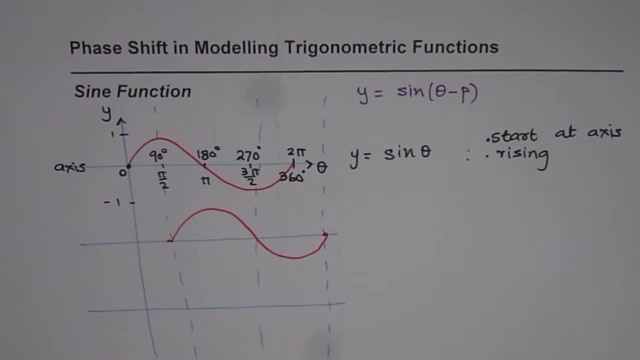 Draw one sine wave right, so Concentrate on these points. So now the same theta we have correct, Xs is same, which is along the x axis, Which I am treating as sine theta. the independent variable amplitude Remains still plus 1 right, same amplitude. 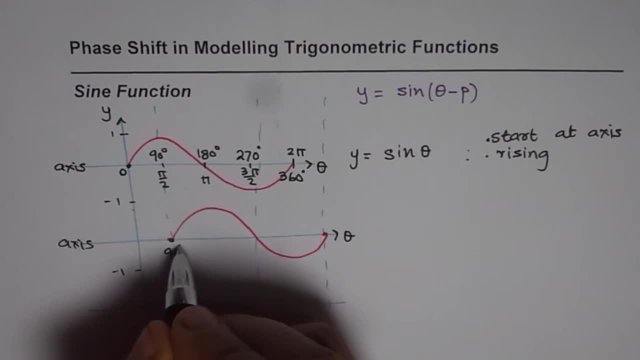 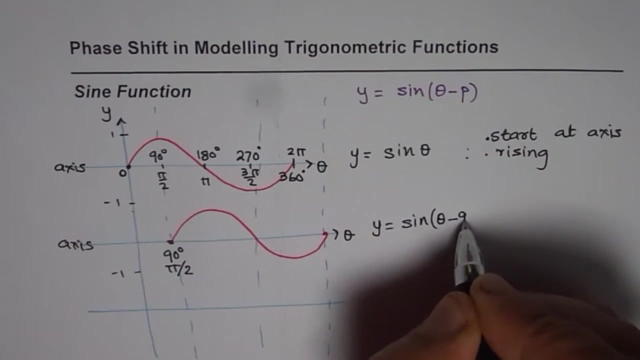 But now the starting point is at 90 degrees, to see, or if you are doing in radians, it is pi by 2, So the equation for this will be: y equals to sine theta minus 90 degrees. for those of you who want to write it in degrees, 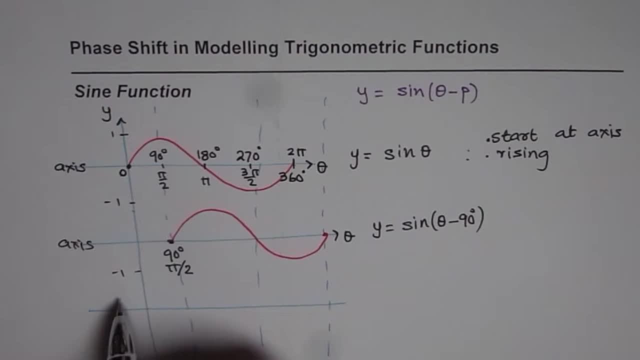 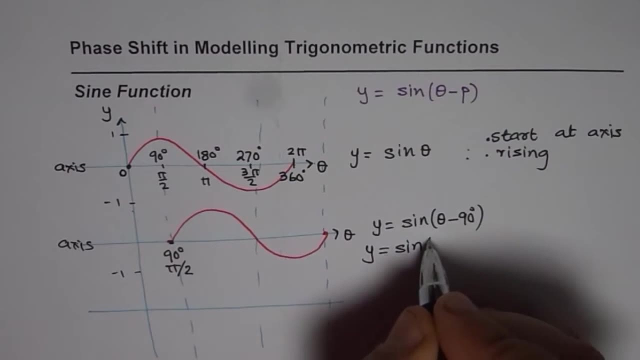 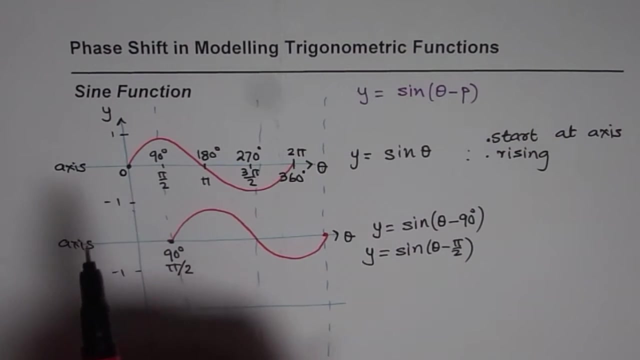 Since it has moved. the starting point of the sine wave Has moved right by 90 degrees in radians. You could write this as sine theta minus pi by 2, right, So that is how you have to incorporate the phase shift. The other condition could have been that this starting point was before right. 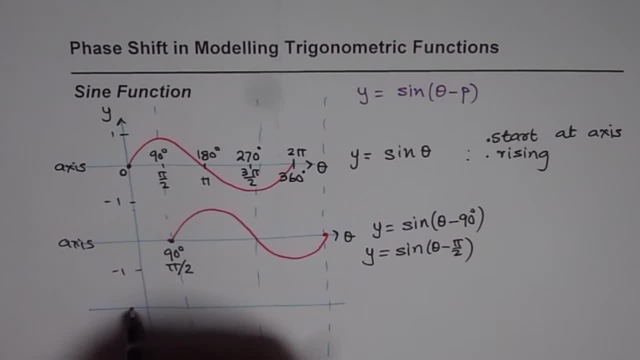 For example, it could be from somewhere here. So let me just draw one wave here. So again, I'm doing very approximate sketch, right? So kind of like this: and let us say that this point here is Minus 45 degrees. okay, 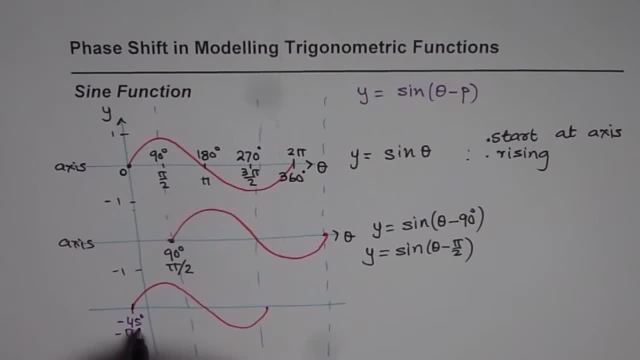 In radians. of course, this would be minus pi by 4, right, I'm taking both the units. now you need to write down the equation for this sine wave, whose maximum is 1 and minimum is minus 1 and whose time period is 2 pi in radians, or? 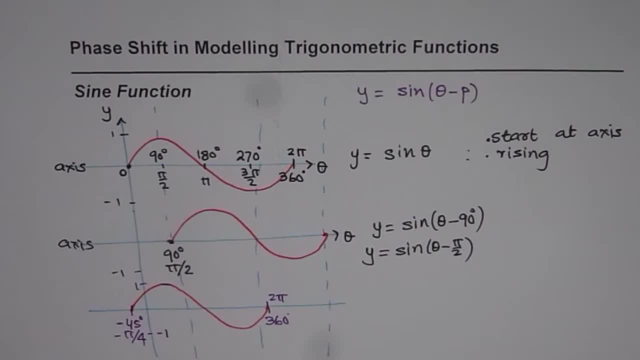 360 degrees. Can you write it? The equation should be: y equals to sine Theta, minus or plus. we have moved left. so minus 45, minus and minus makes it plus, so it'd be plus 45 degrees. or It could be also written as sine of theta plus pi by 4.. I 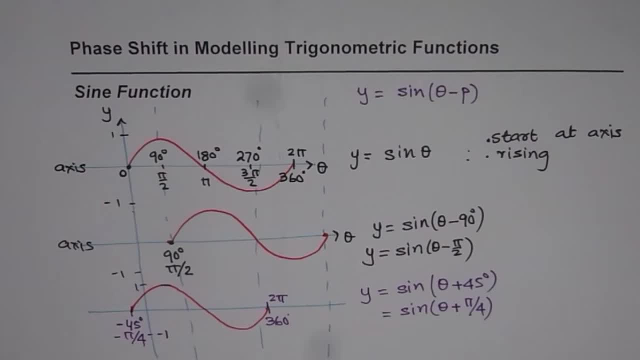 Hope you get it right. So that is how you have to integrate phase shift. Now here is one more suggestion. So this is the last example here on this page. There could be cases when you see the sine wave which actually starts from the origin, But it is not rising, but it goes down first. 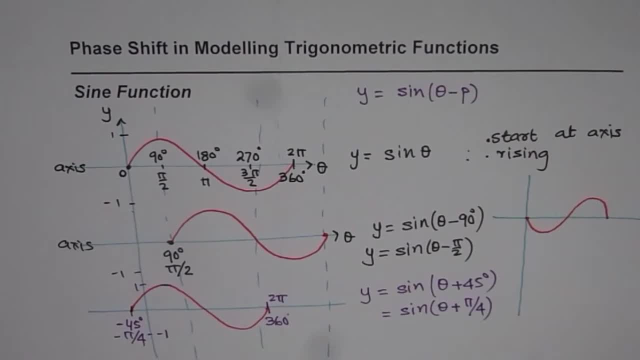 Kind of like this right now. can you write down equation for this sine wave? still, let's consider 1 and minus 1, 2b, its maximum and minimum values and the time period of 360 degrees, or pi, Depending on what units you are taking. 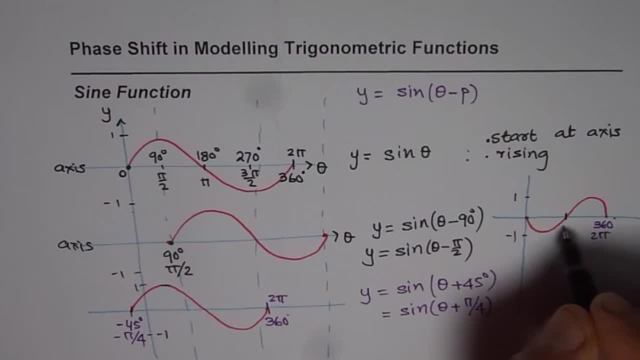 So I mean 2 pi. so half of the wave is that pi or 180 degrees, Is that okay? How will you write equation of this sine wave? Now there are two ways to do it. one is we are looking at a starting point on the X's. 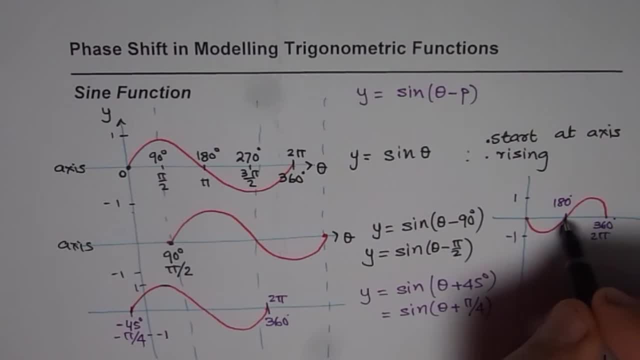 this is the X's and, and rising. if you see, that starting point is really here, so it starts from here and rise, and of course these are periodic waves, so they actually continue, correct? so one way is that i could write this as y equals to sine theta. since it has moved pi or 180 degrees to the right, it'll be minus 180.